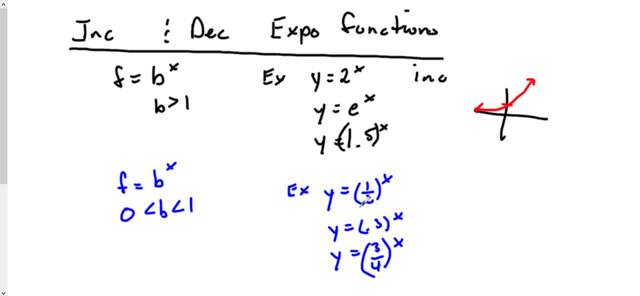 Anything where the base is less than- or sorry, less than one, greater than zero, you have a exponential. Once again, you still have a horizontal asymptote at zero going down right here, but it's going down. So what you're looking for, as the popular song is, it's all about the base. the base, not the exponent. 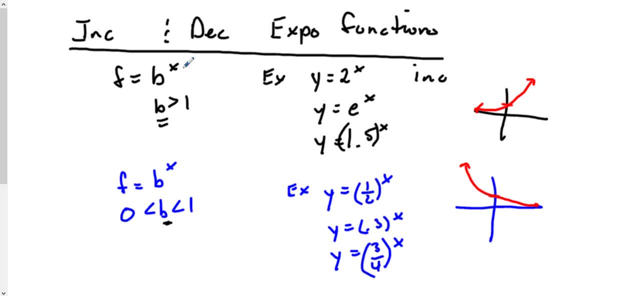 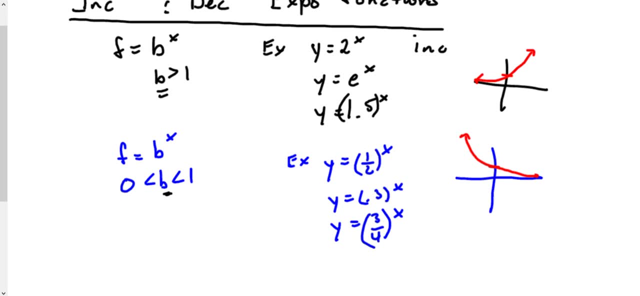 It's all about the base. the base, not the exponent necessarily. However, be mindful that you can also, just so you know, these are decreasing exponentials, decreasing All right. However, be conscious of what is happening, because if there's a reflection, that also changes the increasing and decreasing exponential properties. 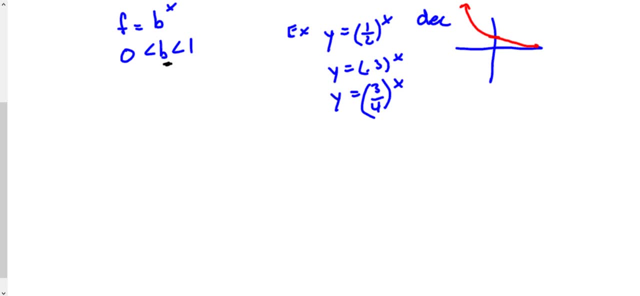 For example, if I have, all right, a base which is greater than one, All right, However, I reflect it, Okay, I reflect it anyway. So if I go and reflect it, any type of reflection will make it the opposite. 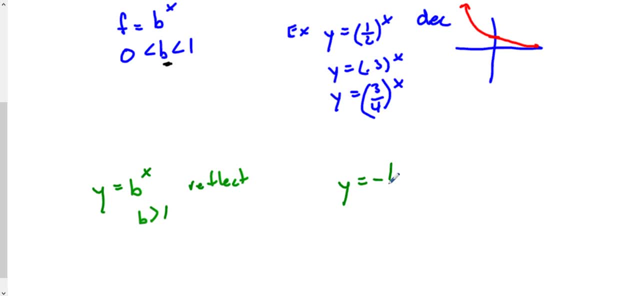 So if I have y equals negative b to the x. what happens is that this graph, instead of going up like this and increasing, it's going to be reflected over the y And this is going to be reflected over the y. So now it's going to go like so: 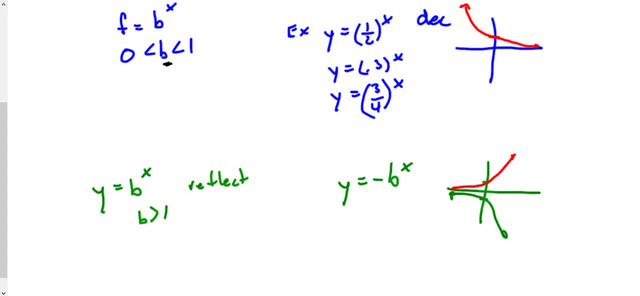 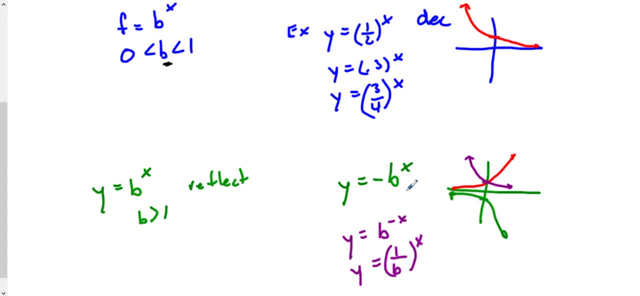 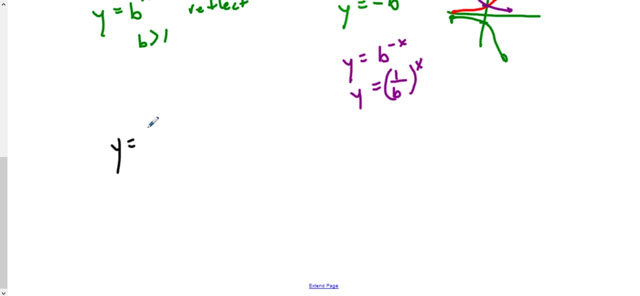 Let's see decreasing exponential. so when you have reflections, it changes to the opposite of what your original base would be, just to kind of show you. and inversely, if we have the base which is X or B is less than 1, greater than 0, all right and you?